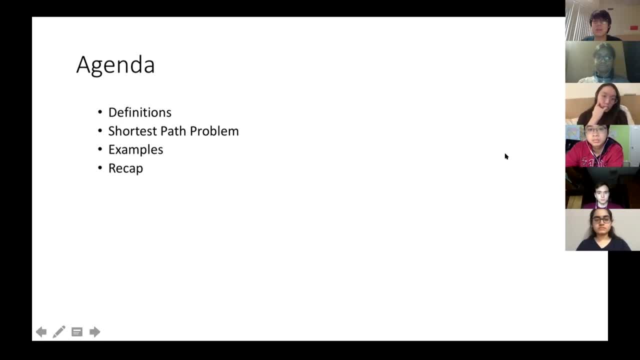 And next we are going to explore one of the most interesting questions in graph theory, which is the shyness pad problems, And then we are going to see some examples and we are going to recap it at the end. All right, And also feel free to interrupt me with any. 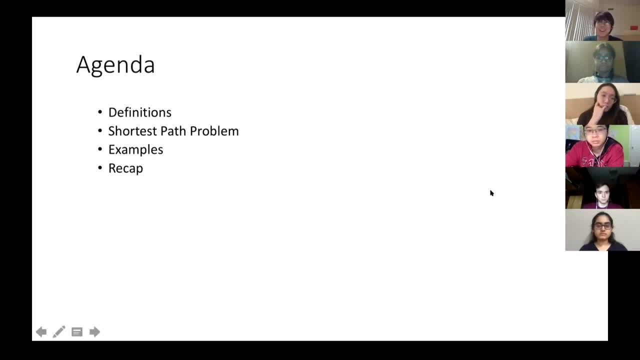 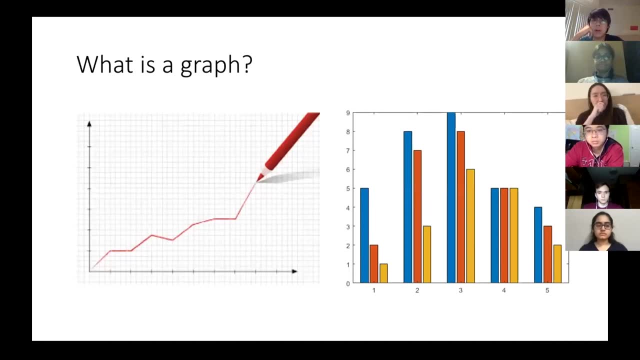 questions you may have. Just don't be shy, Okay. All right, let's dive in. The question is: what is a graph? If you have been dealing with data before, you might have been familiar with the concept of graph. On the left one, you have the graph on the x-axis. 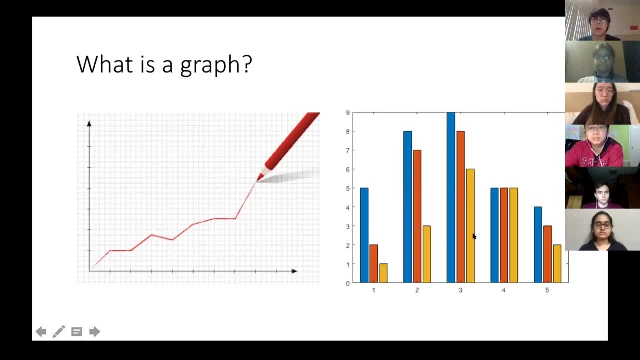 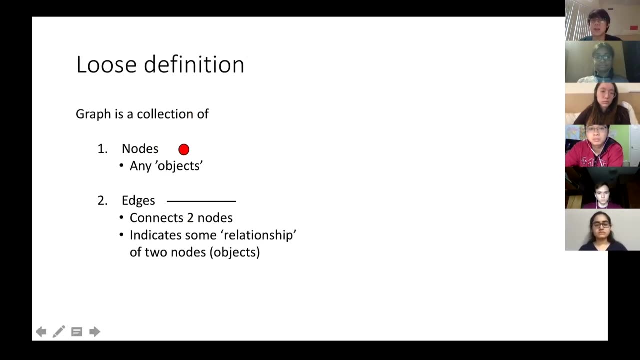 and y-axis, And the right one. you have a bar graph to represent some data, But this is not the graph we are going to talk about today. What we are going to talk about today is quite a little bit different, And the definition of it is: the graph is a collection of nodes. 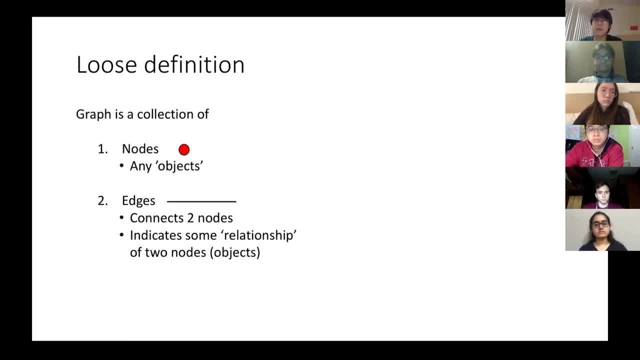 and edges And by nodes. here I will use the red surface And we will be using the. since it has been changed And you can see the graph has changed. The sedative is changed, The circle to represent a node and the edges will be this, just a straight line. so 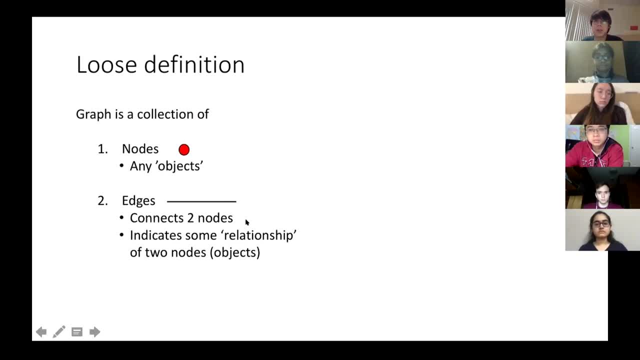 basically, nodes can represent any objects, it can be people, it can be animals, it can be just just anything and the edges will indicate some relationships between two nodes and that might not sound clear. but let's take a look at some examples. yeah, okay, here I have a node that represents Howard and 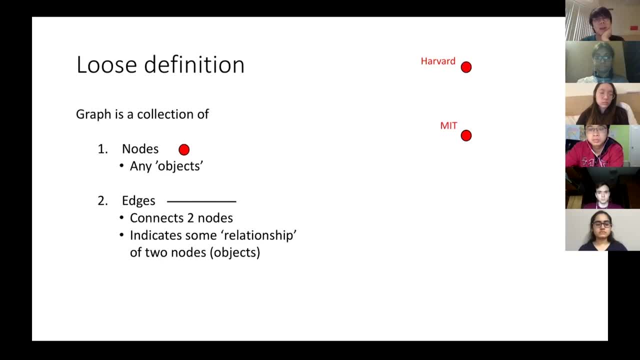 I have a node that represents MIT and they both can be connected by the edge that says they are in the same city of Cambridge. is it clear on this one? yes, all right, and I can have the nodes of Matt and EECS and both are the department at MIT. 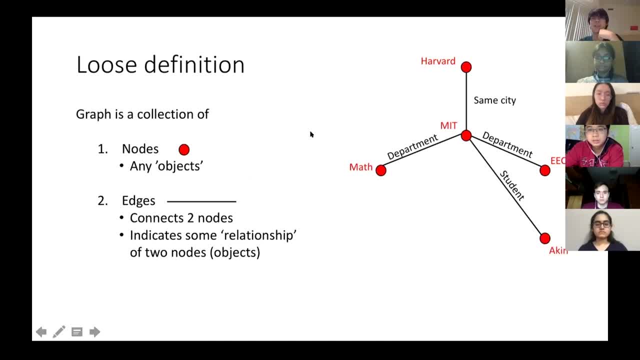 I have a kin. this is me. who is the students at MIT and I study math and EECS. I can have Alice, who loved math, and Bob, who hates math. and listen, Bob, our rival. is it good, okay, uh, okay. I would like to make some notes here, that this 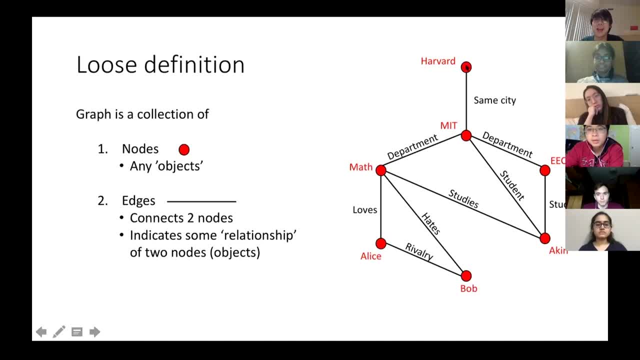 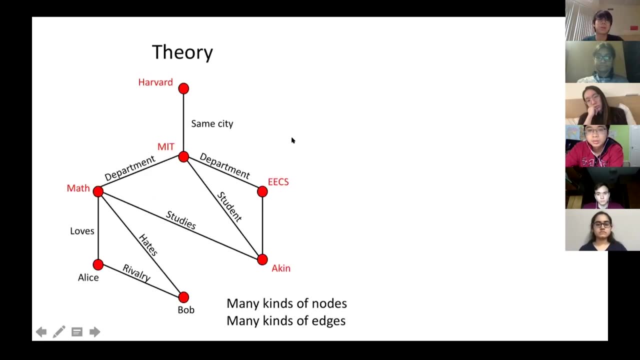 graph is actually quite messy. it has, like, so many kind of nodes. you have schools, you have departments and you also have people, and in the same time you also have so many kind of ages. you have the same CD as department students and many more. so, in theory, 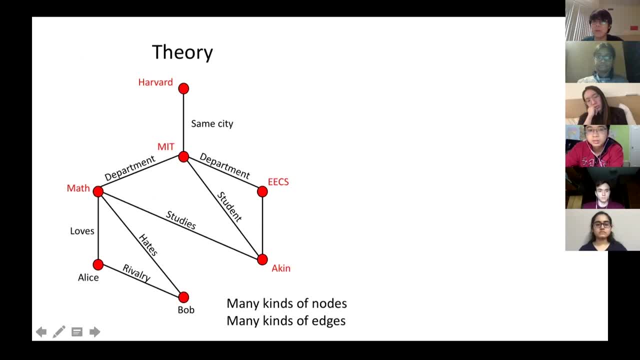 this is not wrong. in one graph you can have so many kind of nodes and so many kind of ages, but in practice we usually refer to a graph as only having one kind of nodes and one kind of ages, and what it means by that. if you take the 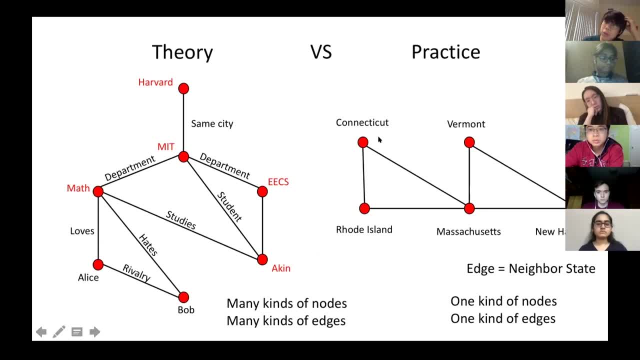 look at the right graph. you can see. this graph has nodes that are the states in New England and the edges is an indication if two states are neighbors. Are these still on the same page? Yeah, and this is. I also have some examples so you 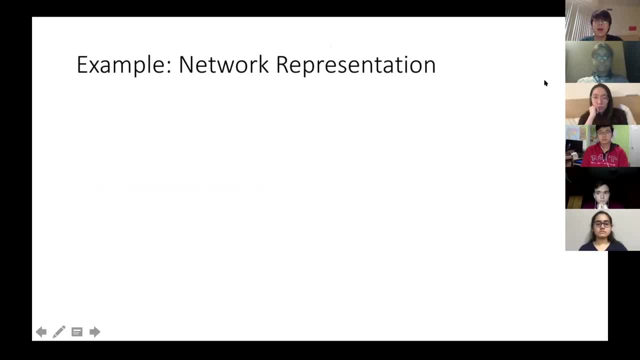 can probably have a better understanding. The example I'm going to use is the network representations, and probably you guys have seen Facebook before And what we are going to do is Facebook actually have a very nice way to present the network as a graph and to do so you can have the node to represent a user and 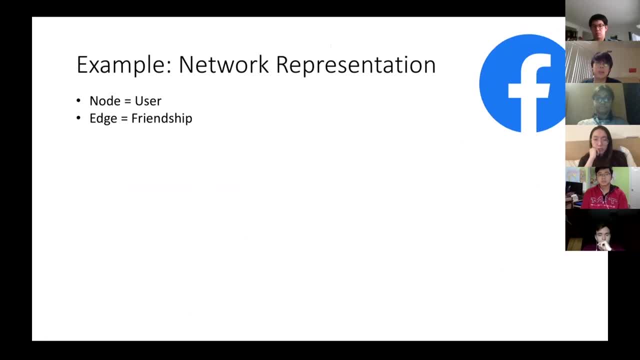 edge to represent the friendships between any two users. For example, this diagram: here you can see a list here. List has edge that connects to Emma, Shane and Alan. That means list has three friends, which is Emma, Shane and Alan. Is it okay? Yeah, okay, I just want to ask, like to make. 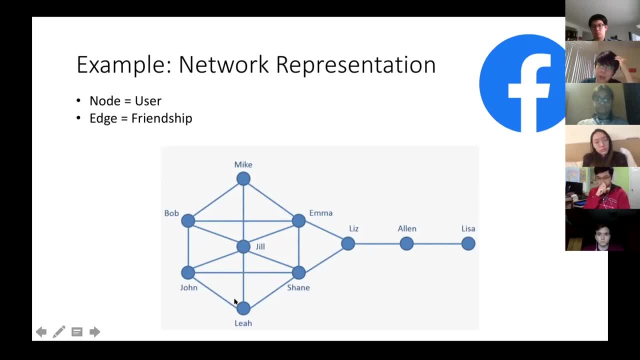 sure everybody is on the same page. like just a quick question like: how many friends does John have? Four, Four, yeah, Yeah, there are four friends of John: Bob, Jill, Shane and Leah. Okay, still good. 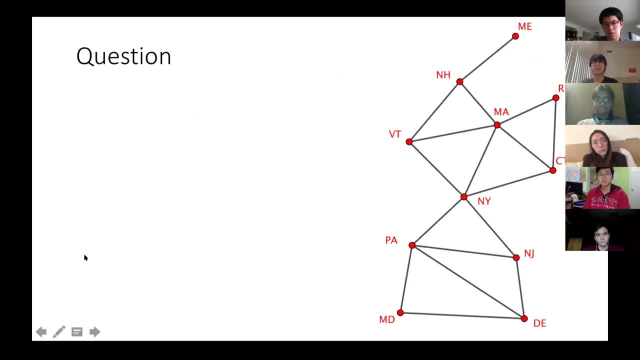 Okay, Okay, I have another question for you. On the right. I have a graph whose nodes are some states in the US. You can have Maine, New Hampshire, Massachusetts and many more, And the edges will represent that there is a road that connects two nodes together. 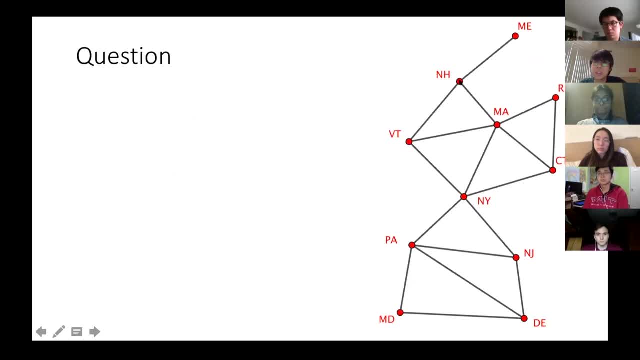 For example, this edge is a road that connects Maine and New Hampshire. This edge is a road that connects Vermont and New York. So basically, you can view this graph as a map and there are states, then there are road that connects states together. Yeah, So here's my question. 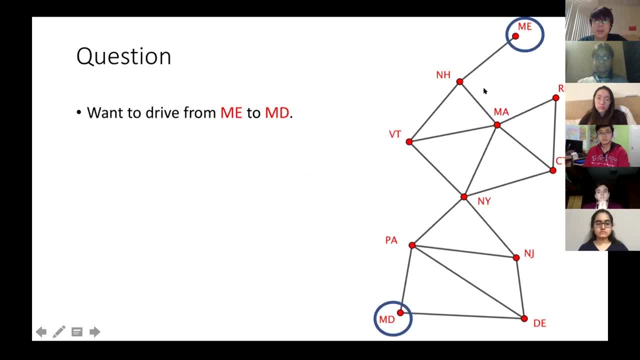 You want to drive from Maine to Maryland. Yeah, Okay, Okay, Okay, Okay, Okay. So you want to drive from Maryland, which is this circle, to this circle and to use a road. you need to pay $1 for each road you take. Yeah, The question is that, what is the? 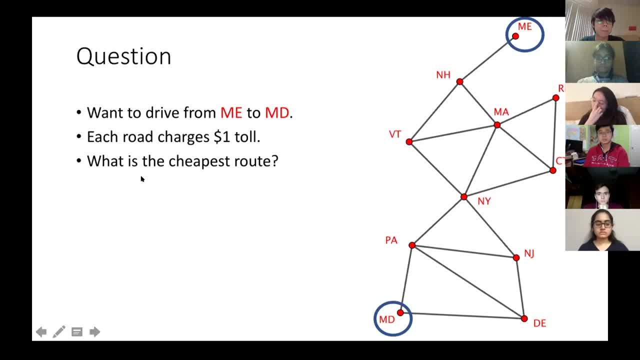 cheapest route. you can take Any figures. No, You can go along to the left edges. Left edges, you mean, Yeah, New Hampshire, Vermont, New York, Pennsylvania and Maryland. Yeah, yeah, that's perfect. There are actually two sheet-paste routes here, which are indicated by the green lines. 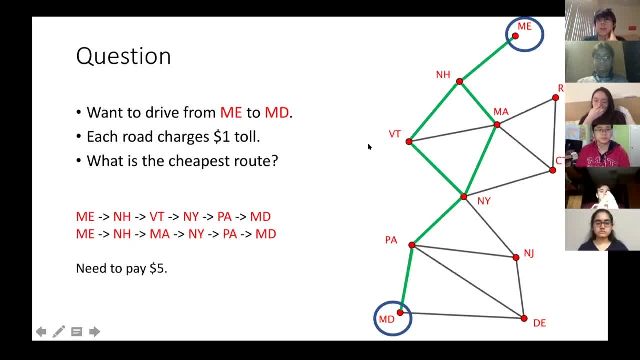 Whatever route you take, you need to pay five dollars, And this is what we call the shortest path problem. I will explain it in a minute. but if you guys have any questions, if you don't understand the graph, you can ask me. 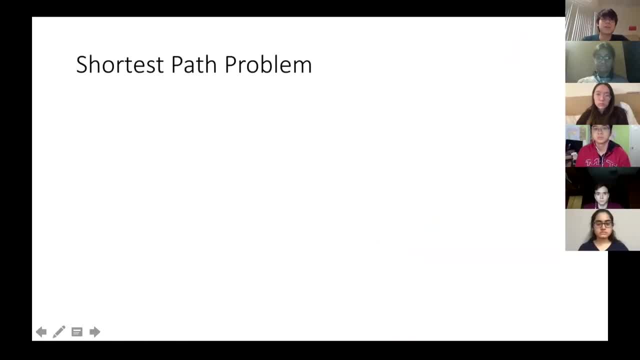 Okay, let's move on. So the shortest path problem. It is probably one of the most important questions in graph theory. Computer scientists have been dealing with it for decades and it also has so many applications in real life, And the way we formulate a problem is that we are given a graph. 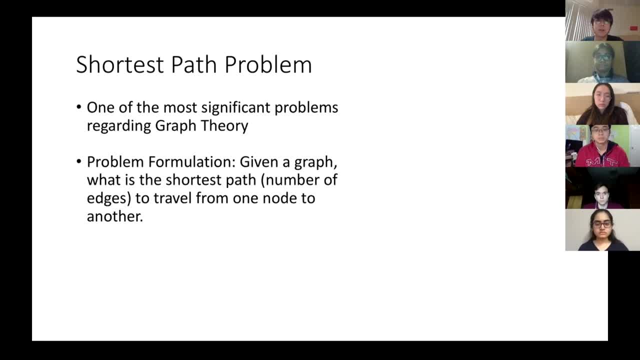 and we want to find the shortest path in terms of the number of edges to go from one node to another, like we just did to go from Maine to Maryland, And it's actually easy to solve by eyes if the graph is so small, like. 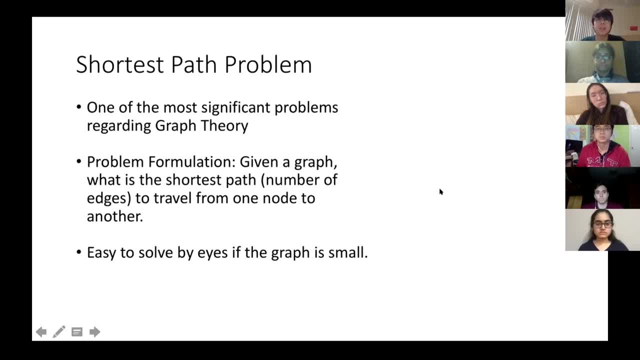 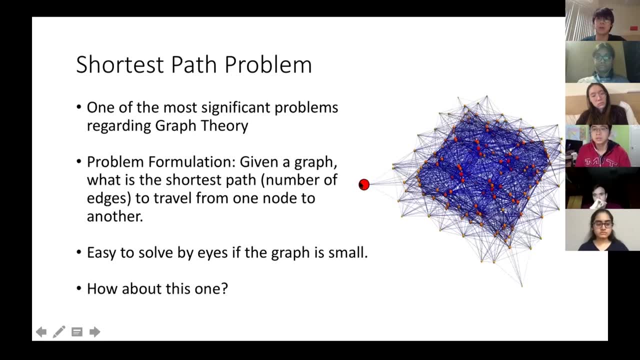 Nikita? did I pronounce correctly? Yep, Yeah, he just solved it in like 10 seconds and it's pretty easy if the graph is small. But the question is like, if the graph is large, how do we do it? Like on this one. 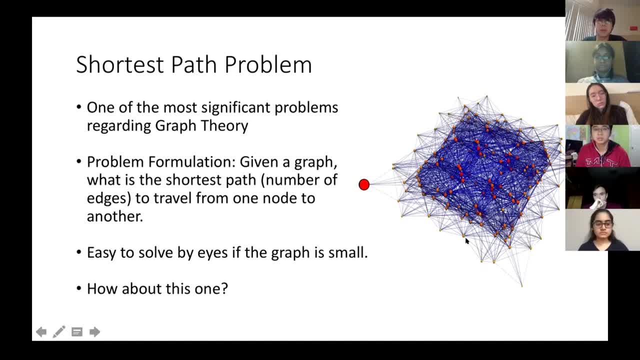 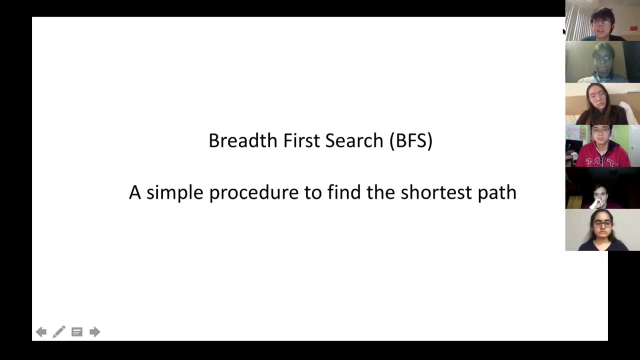 if you want to go from the left node to right node, it's probably impossible to solve it by eyes because you know there are like 100 nodes and 1000 edges. So to solve these problems, computer scientists have come up with a very nice and very simple procedure to find a shortest path. 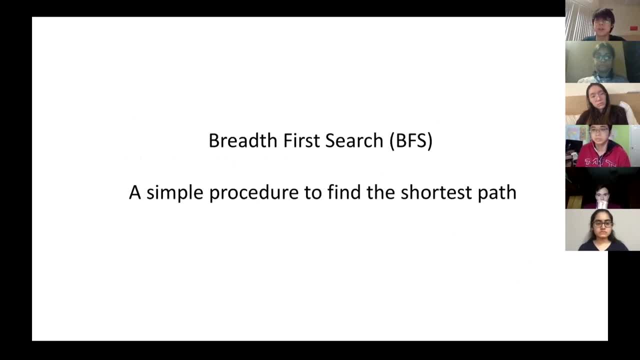 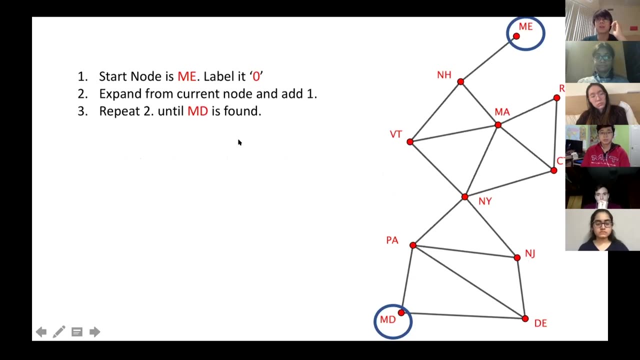 And we call it the Bread First Search, or BFS for short. And we are going to do it now and I'm going to list the instructions on the left and we are going to solve it together on the right. So to do it, we are going to start with. 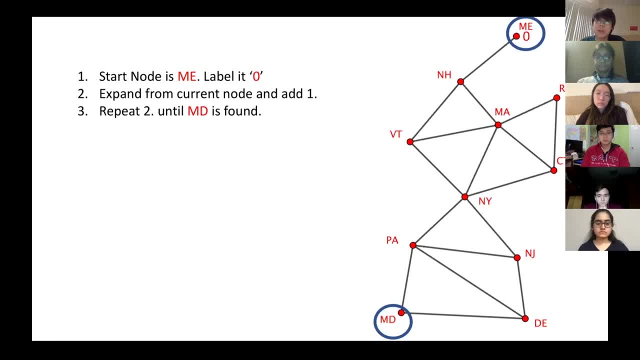 labeling the start node, which is Maine, here with 0, and then we are going to see that from Maine you can expand to New Hampshire. So we are going to put 1 at New Hampshire and then from New Hampshire you can only go to Vermont and Massachusetts. 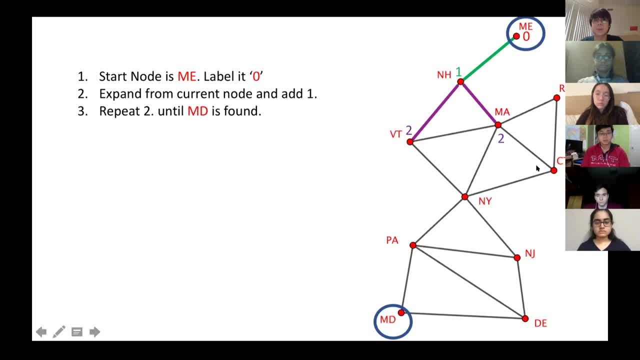 So we will put 2 here, And if you do the same thing from Vermont and Massachusetts, you can only go to New York, Connecticut and Rhode Island, and we'll put 3 there. And we are going to do it again and again until we find Maryland, which is 5.. 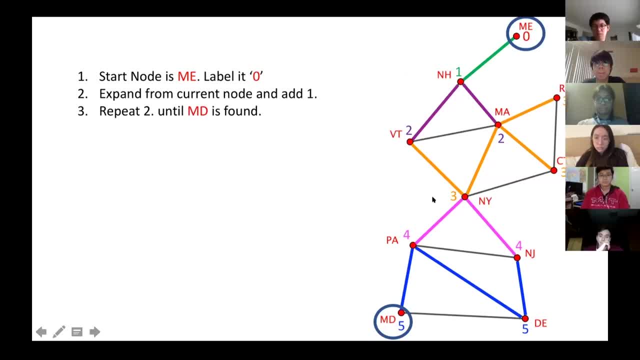 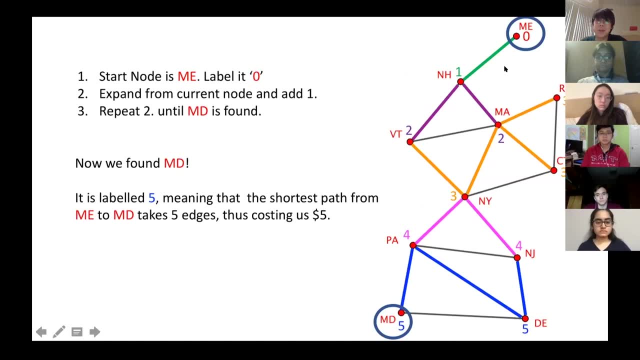 Is it clear on the procedure? Yeah, Yeah, Sounds good. Okay, So we found Maryland. it's level 5, meaning that to go from Maine to Maryland, you need to take 5 ages. However, these procedures only tell you the least number of ages you need to take. 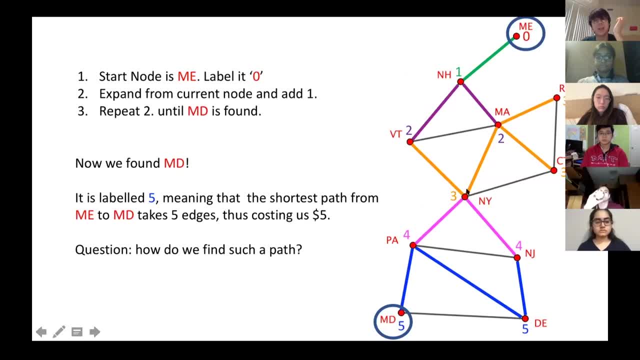 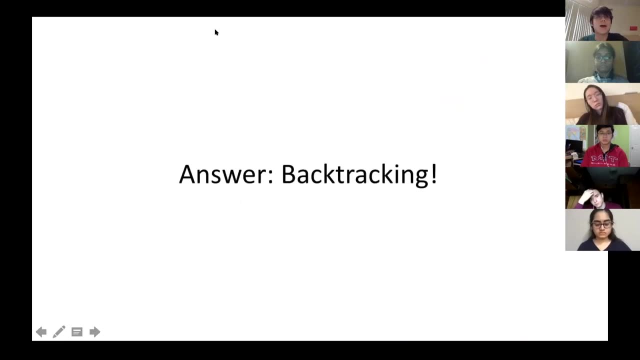 but it doesn't exactly tell you what path you should be taking. So the question is: how do you find such a path that costs you $5?? Okay, Well, you will obviously need higher level roads based on your transfer in the residential化, and you need access to the knowledge about Are. 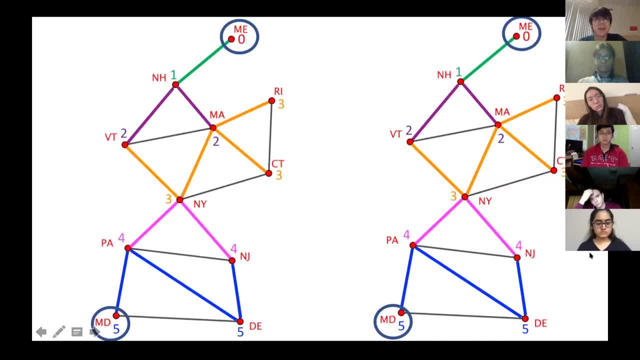 And the answer is what we call Back Tracking, And it is quite simple too. So what it means by backtracking is that you have Maryland at 5 and you have Maine at 0.. You want to find a path that goes, uh, 5, 4, 3, 2, 1. 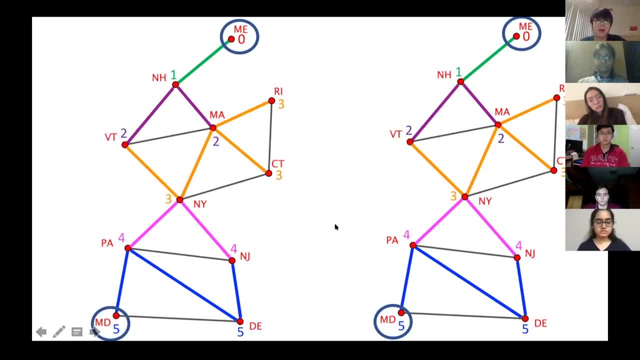 and 0.. and to do that on the left one you can go 5, 4, 3, 2, 1 and 0, And if you follow this, where you can see that you have Maryland at 5, and you've Maine at 0,, 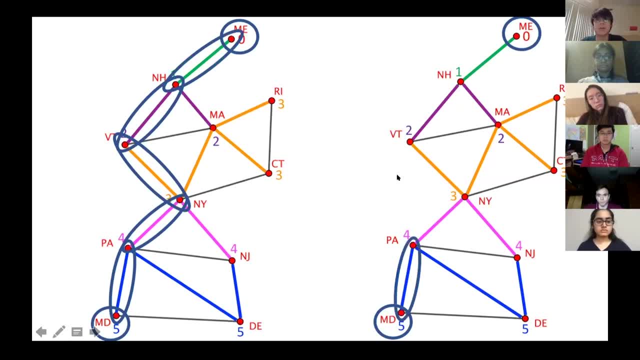 You want to find a path that goes 5, 4, 3, 2, 1, and 0. And on the right one you can go five, four, three, two, one and zero, And these are actually two paths that we just solved earlier by eyes. 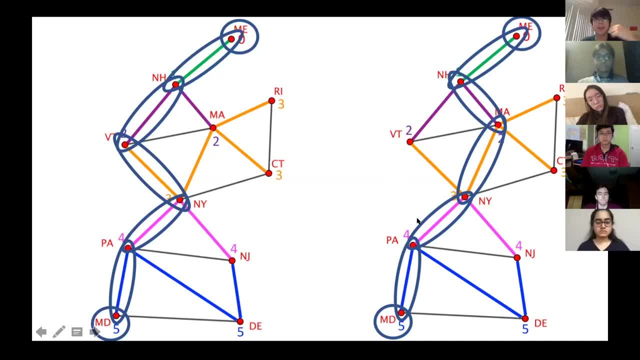 Is it clear for everybody? Yes, Okay, Sounds good. So how do you guys feel about this example? Is it like too hard, too easy, or just okay, It's all right? It's all right, All right, everybody. 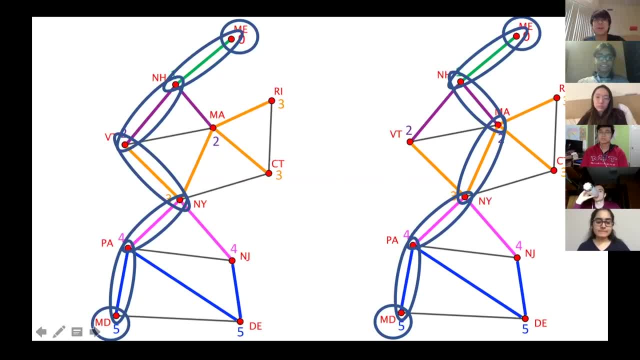 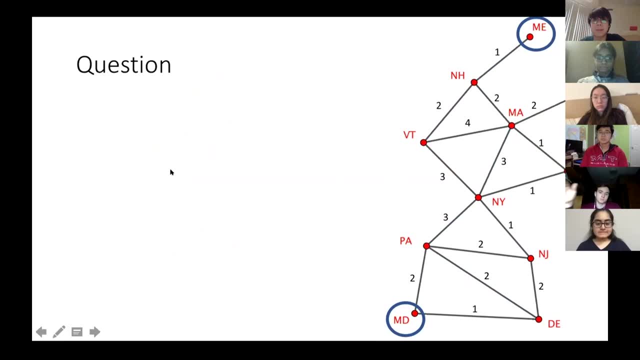 Okay, if this is not too hard for you, I have two questions that might be a bit more challenging. For this one, you still have a map. You have to have the same graph with the nodes of the states, But now each road will cost you differently. 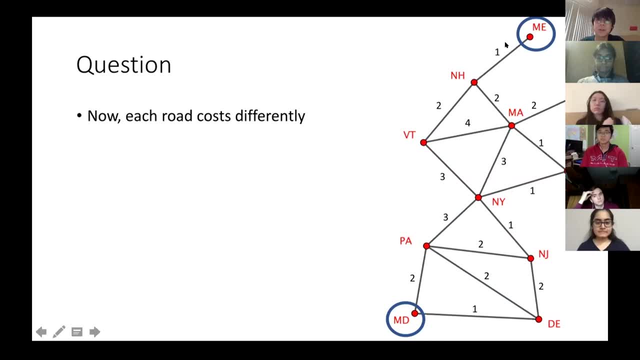 Like, for example, from Maine to New Hampshire, it will cost you $1.. And from New Hampshire to Massachusetts, it will cost you $2.. So basically, like the numbers above the eight, it should tell you the amount of money you need to pay for using the road. 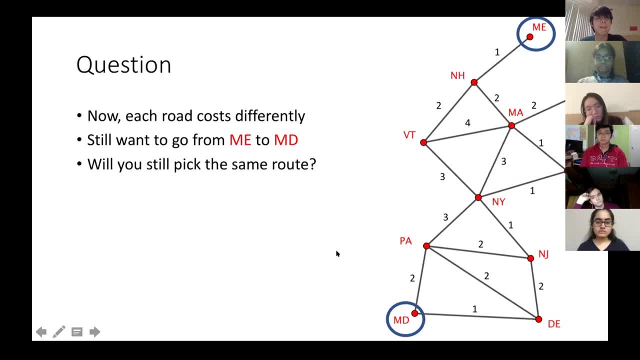 You still want to go from Maine to Maryland, but you still pick the same route. I will tell you here that the old one will cost you $11.. Like one, two, three, three and two. Yeah, can we do better? 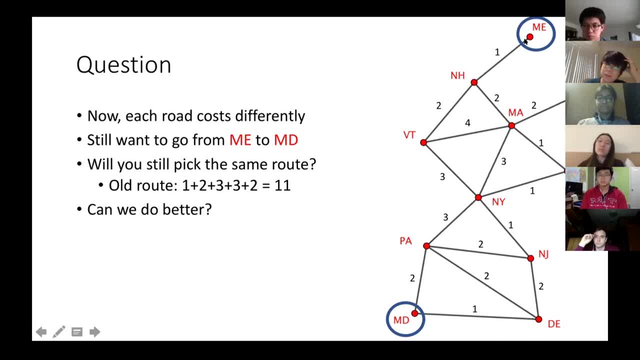 I think in the lower part of the graph we can take the right route this time. So it would cost $4.. Yeah, Yeah, that's a good cash. You could go this way. You only need to pay for it, right. 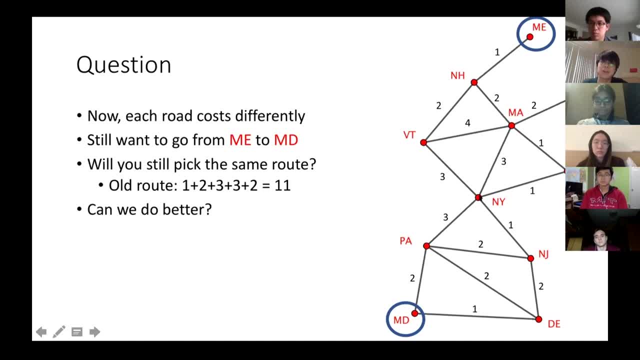 How about the upper part? And you just find the charter way, The cheaper way. Okay, Okay, Okay, Okay, Okay, Okay, Okay, We can go from New Hampshire to Massachusetts, to Connecticut, to New York. Yeah, Yeah, that's correct. 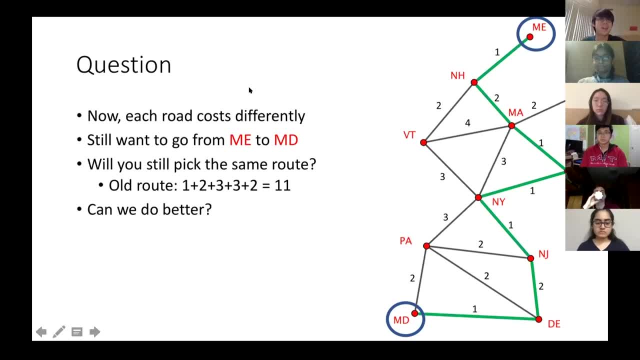 And this is actually the cheapest path we can find. So this type of question, we call it the weighted shortest path problem. It's basically the shortest path problem with some variations. So here every age will have the corresponding weight. In this case the weight is just the amount of toll we need to pay. 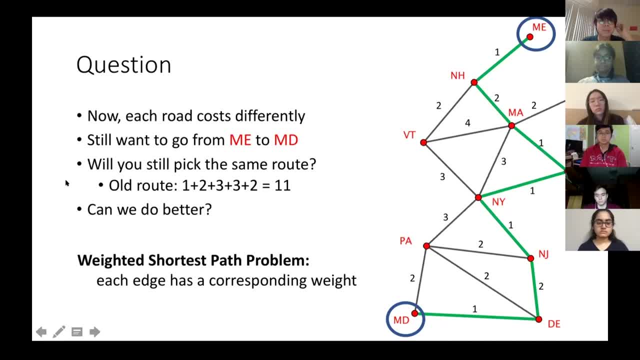 Okay, Okay, Okay, Yes, I peut kan unserem by using the row. Is everybody still good? Okay? So, as you can see, the traditional breakfast search. do not work on this graph, because it would just tell us to go on this way, the old way, but the actual cheaper route is just. 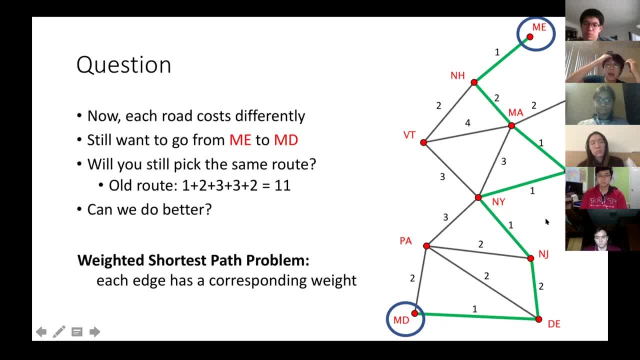 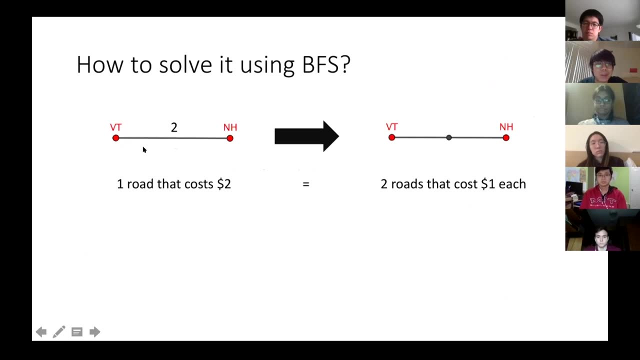 to go on the green line. So the question is: how can we solve it? By using the BFS? Uh huh. The answer is we need to do some modifications To use the VFS to solve it. we can add an intermediate node here. 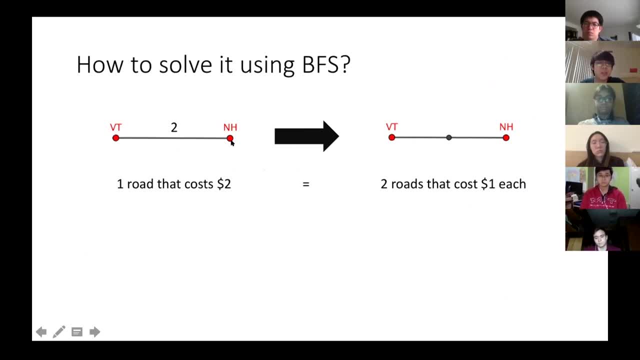 So we're basically going to split up the roads. So from one road that costs you $2, it's going to be split up into two roads that cost you $1 for each road. Is the diagram clear for you? Yes, Yeah. 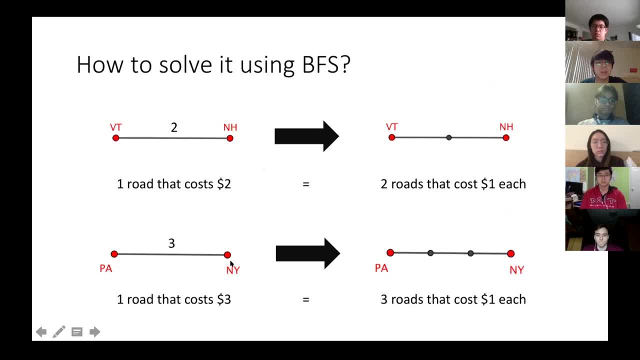 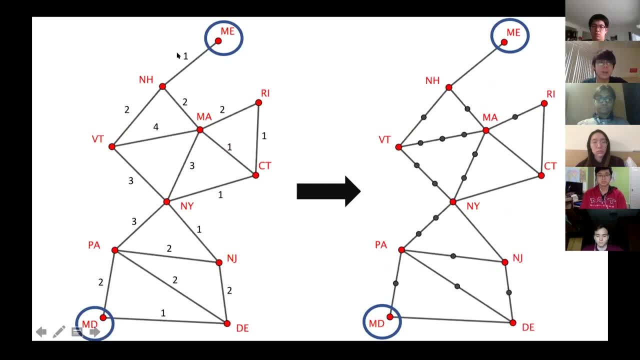 And also the same thing with the road that costs you $3 can be split into three roads that cost you $1 each, And you can transform the graph from the graph with the weights to the graph with intermediate nodes. As you can see, Massachusetts to Rhode Island: $2 will be split into two roads and you can 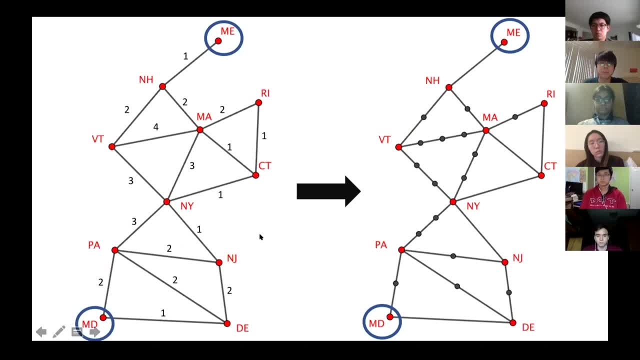 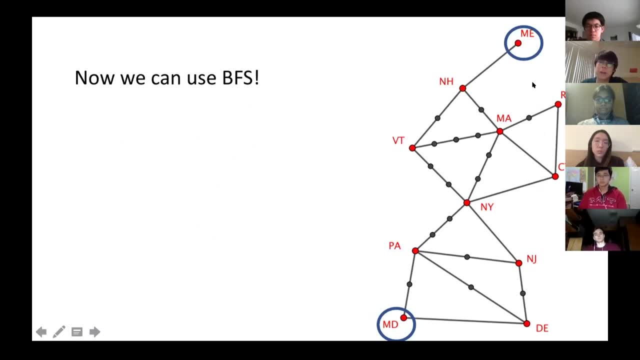 do the same for every single age And from here you can use the VFS like we just did before. I'm going to just show you how it goes, because it will take too long. You have 0,, 1,, 2,, 3,, 4,, 5,, 6,, 7,, 8,, 9.. 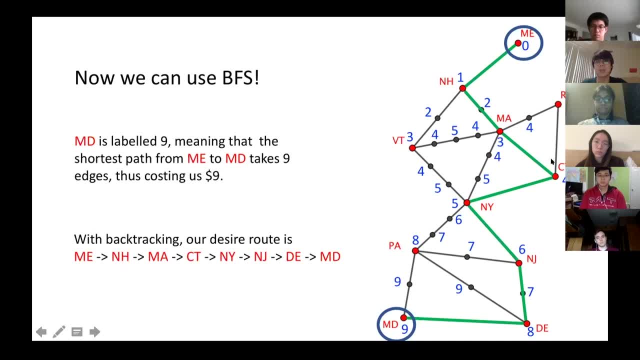 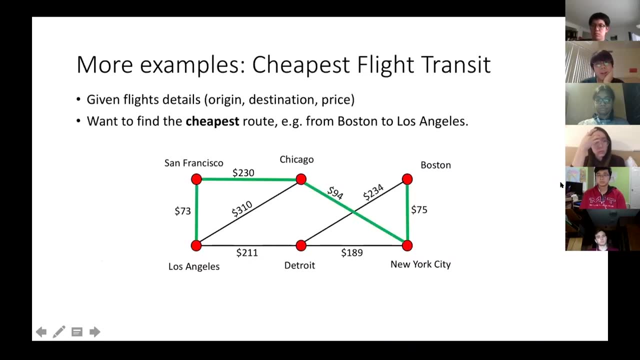 And you can do the backtracking to find the actual shortest path. Is it clear for everybody? Yep, Yeah, Sounds good, Okay, Okay. I would like to end with a couple of examples that you may have come across. So these are the actual examples in real life of the VFS. 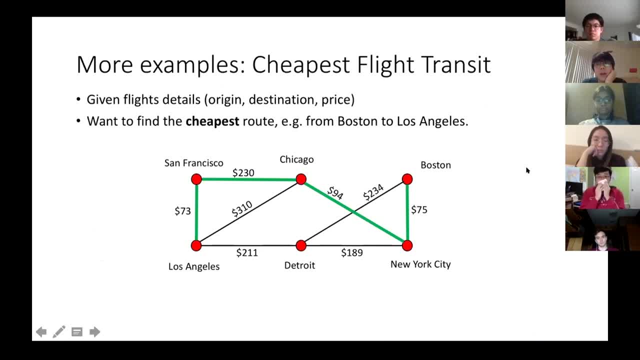 So the first one is the cheapest flight transit. If you have used some traveling agents before, you will want to go from one place to another. But if you do the search, it will tell you what is the cheapest route, what is the transit. 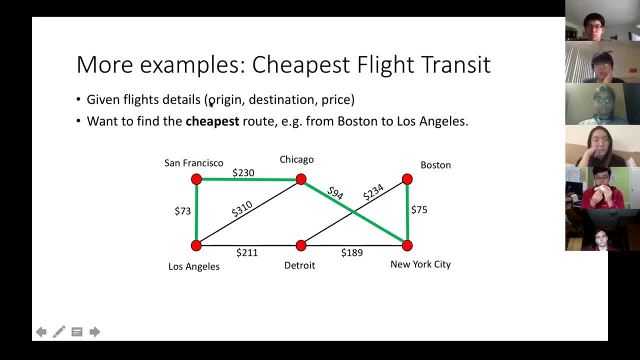 So in this model you are given the origin and destination and price of several flights And for example, here you want to go to Boston, to Los Angeles. You can use the breakfast search to see that this is actually the cheapest route you can. 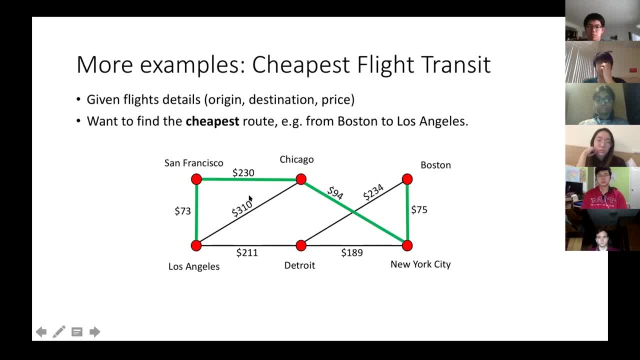 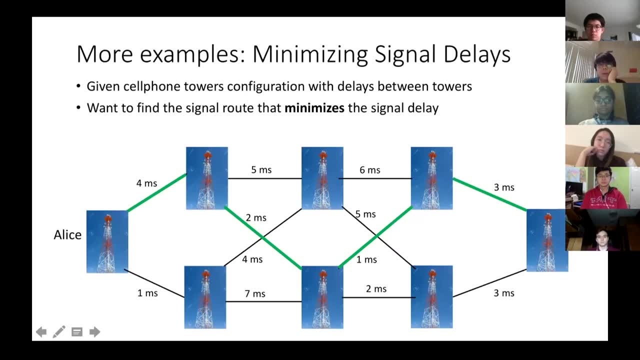 find. And another example that I have here is the minimizing the signal delay. So if you want to call a friend, like at least want to call Bob, want to call Bob, so the signal actually going to bounce off a lot of cell phone towers until you're reaching. 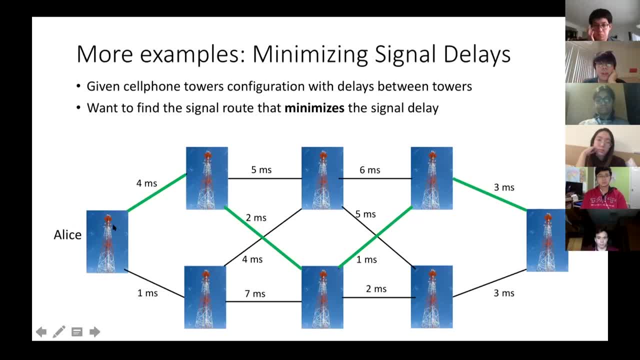 the destination And from the signal to go from one tower to another tower. it has some delays. So we can model this as a graph, with the node to be the cell phone towers and the edge to represent the delays from tower to tower, And we can use the breakfast search to see, like what should be the fast route, that signal. 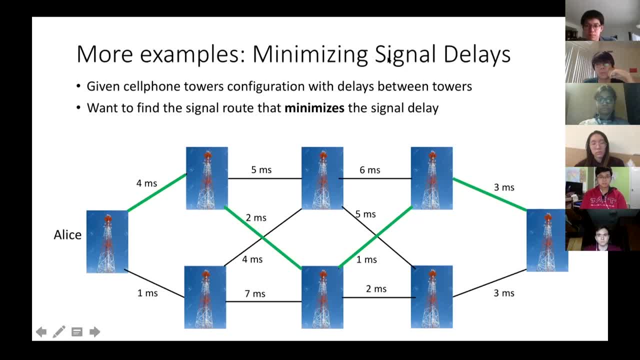 actually minimize? Yeah, Is the example clear to everybody? Yep, Yeah, And that's pretty much all I have for today. Just want to recap everything up. Today we learned what the graph is And we see how to solve the shortest path problems by the breakfast search, both on. 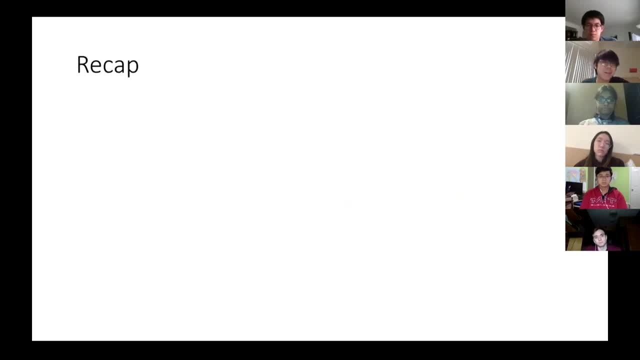 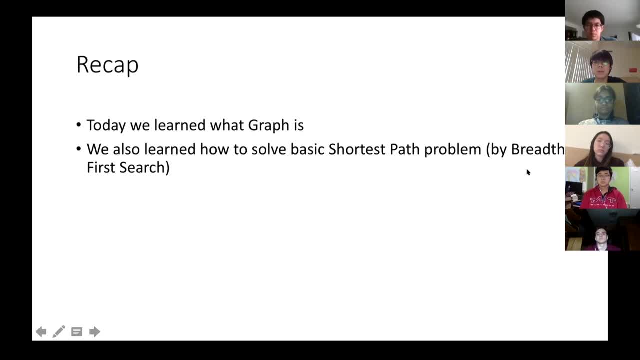 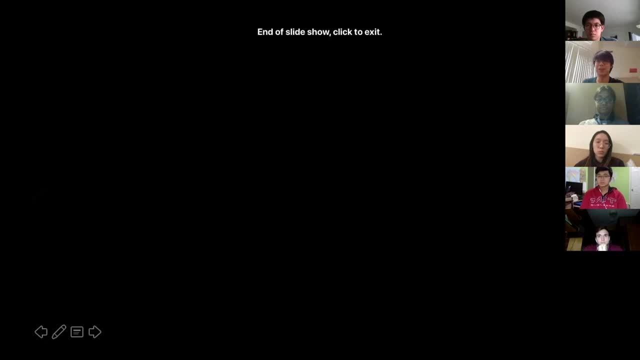 Thank you, That was also my one question. Um, I'm out of time, so we might move the next session on towards the end, but remember you had to do a lot like rule planning and minimizing delay and yeah, that's all I have for today.